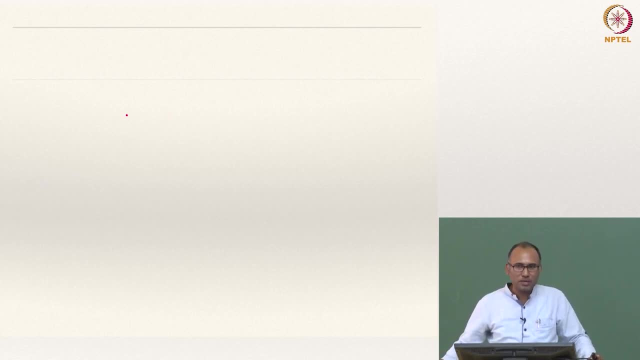 on the chapter name itself is the tension test. You get lots of information, insight into the reason why these curves are the way that they are. So all the discussion that we had in the class you can reinforce by reading the tension test. 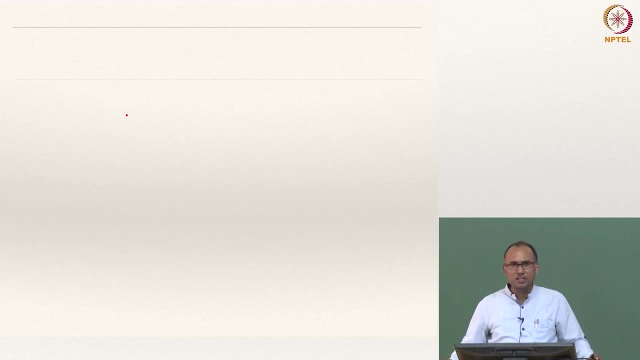 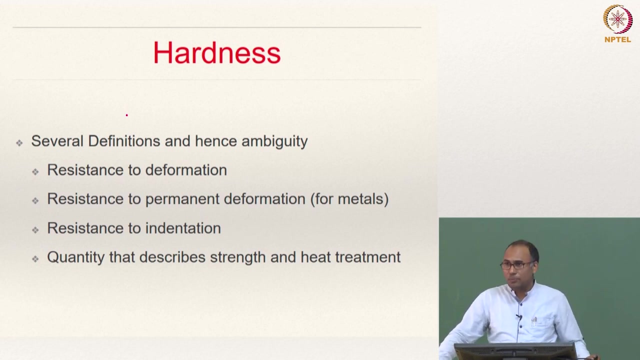 That chapter. it is about 30 to 40 pages, but it is really a worth reading. So then the next property: hardness. and how do we go about measuring hardness? So there are several definitions available in the literature for hardness, and hence it is quite ambiguous. 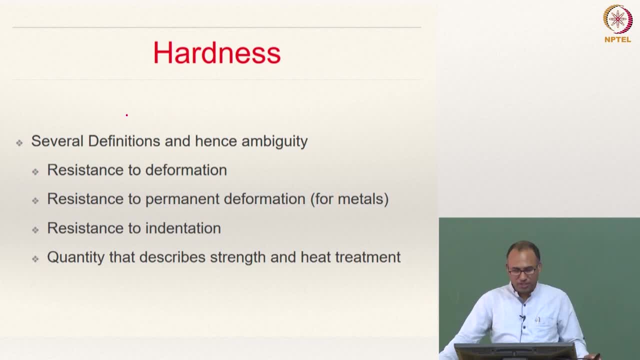 People define hardness as resistance to deformation, Some people define as resistance to permanent deformation for metals And some people define it as resistance to indentation. And somebody says that the quantity is that hardness is a quantity that describes strength and heat treatment. So which one? 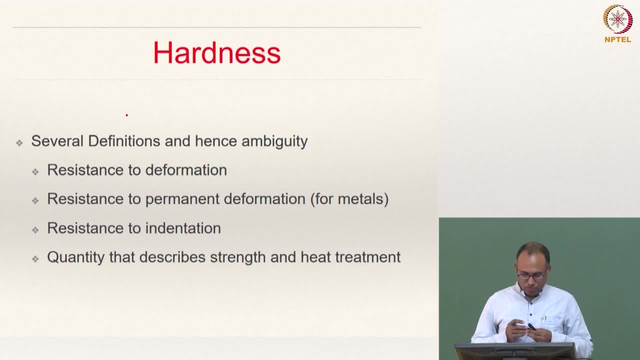 to follow, you do not know. So, because there is lot of ambiguity in this class, we will try to fix to one definition that is more suitable for mechanical engineers. So the definition that is more suitable for mechanical engineers. So the definition that is more. 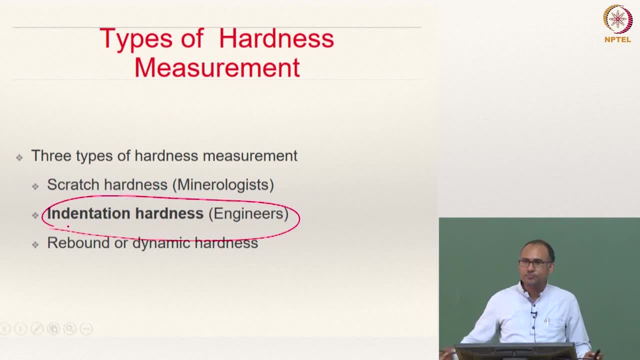 suitable for us is indentation hardness. If you are talking to a mineralogist who is looking at minerals and rocks and so on, for him or her the type of hardness is scratch hardness. What do you do? Scratch hardness means take a sample, scratch it If you are. 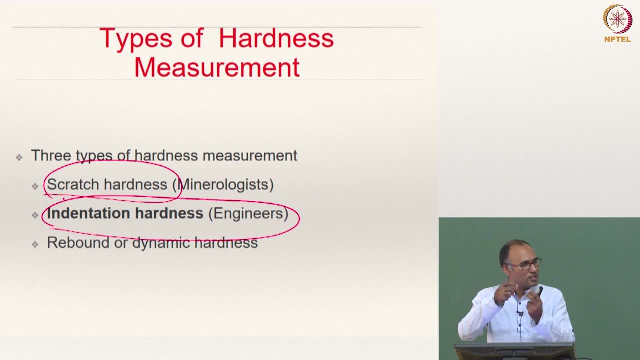 able to dislodge the material, then it is softer. If you are not able to dislodge, then it is harder. Of course, you do not know, So you do not know, So you do not know, You do not do with hands, But they will have some technique to actually dislodge the material. 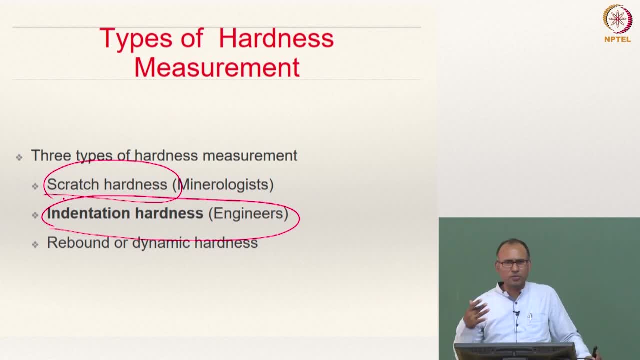 But essentially that is what they do And that is a reasonable way to look at hardness for mineralogists And for us. indentation hardness: That means you take a material and then you indent using a indenter And when you look at the depth indentation- 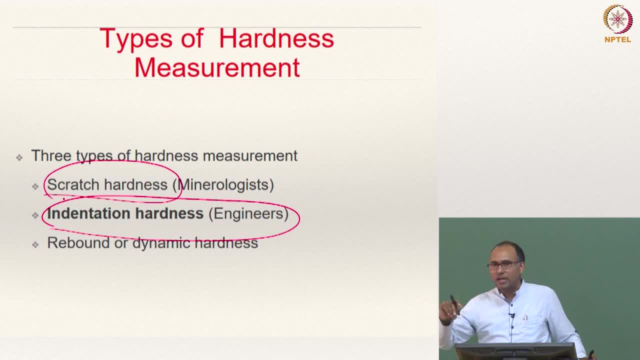 depth. and if it is a hard material, your indentation depth is going to be small. and if it is a soft material, your indentation depth is smaller. If it is big, teeth, bondian, if it is very soft, boobs, So indentation depth is less Inter jet depth because you are making go. 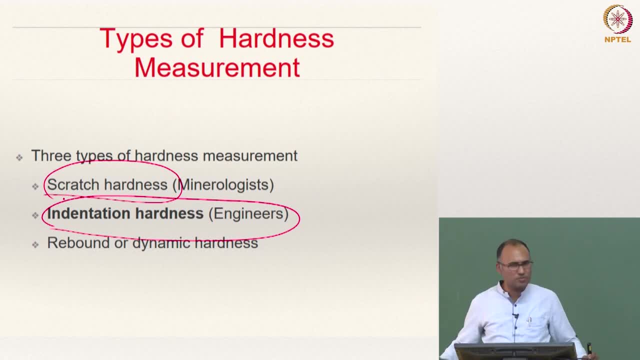 is going to be hard. That is something that we can relate to even without doing an experiment. right, If you take a sponge and if you take a rock, obviously if you indent, the sponge goes in. so that means the depth of indentation is increasing for soft materials. 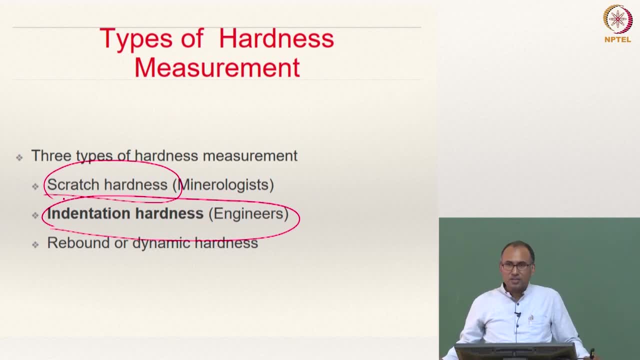 And for some people it can be rebound or dynamic hardness. You take a ball, drop it on a surface and the height to which it rebounds tells you the hardness of the surface or the ball right. It is like coefficient of restitution that you probably have studied right. 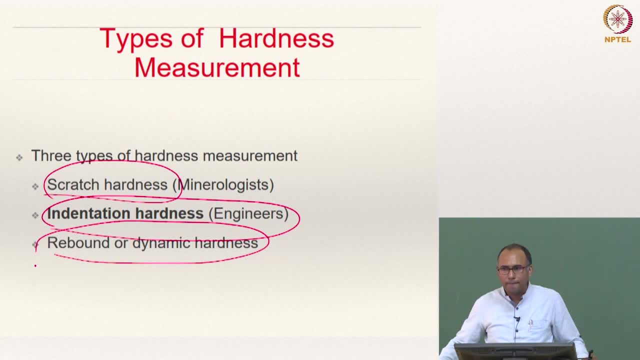 So if it is a very soft material, the coefficient of restitution is going to be higher or lower. So if you take a ball right and bump it on a concrete surface, put a mat on a concrete surface and drop it, You will see the rebound. 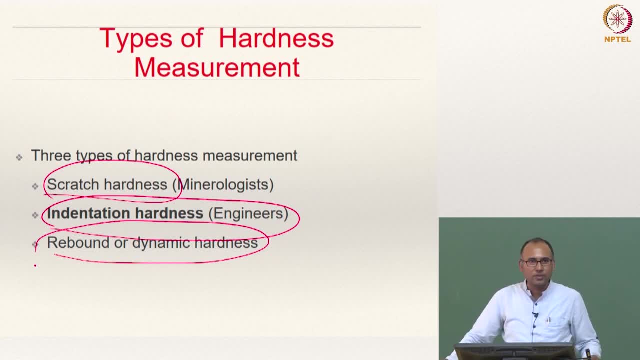 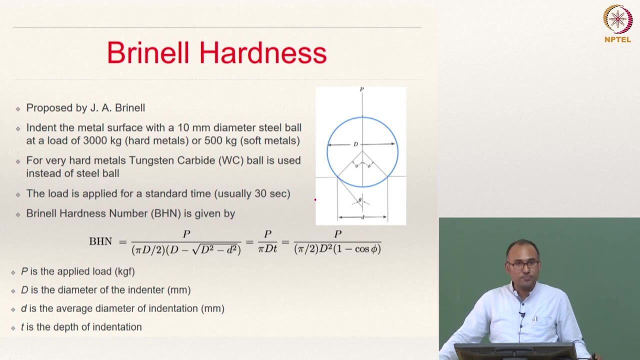 The distance is different, right, That is also another measure of hardness, But in this class let us restrict to indentation hardness. okay, So there are different kinds of test one can do in order to measure hardness through indentation. Now, one of the methods- earlier methods- is what is called Brinell hardness. 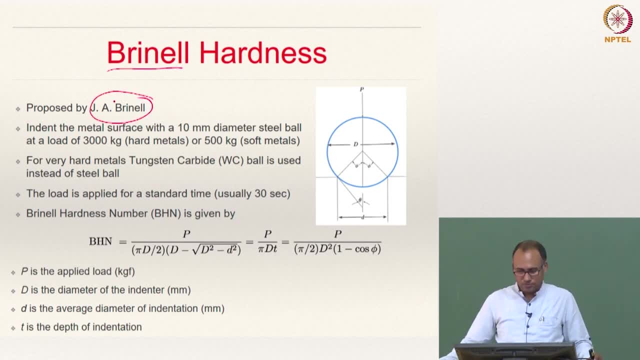 It is proposed by person called JA Brinell. So what is Brinell hardness? So there are some standards, like tension test. uniaxial tension test has some standards. You have to have your specimen of certain dimensions, and so on. 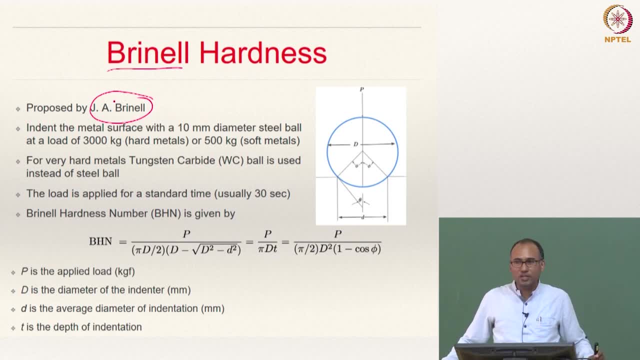 And if you want to change the dimensions- you cannot change the way that you want- You have to maintain some similitude so that your relation, your results can be correlated. So the geometric similitude is important, even when you are doing uniaxial tension test. 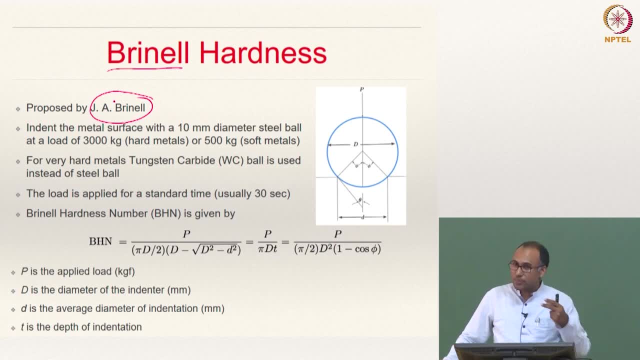 And if you want to change your dimensions from the regular dimensions. that is something, that information you can find out from the Dieter's textbook that I have suggested. okay, Alright, So how do you go about doing this test? You use an indenter and then, using that indenter, you actually apply a load on to the surface. 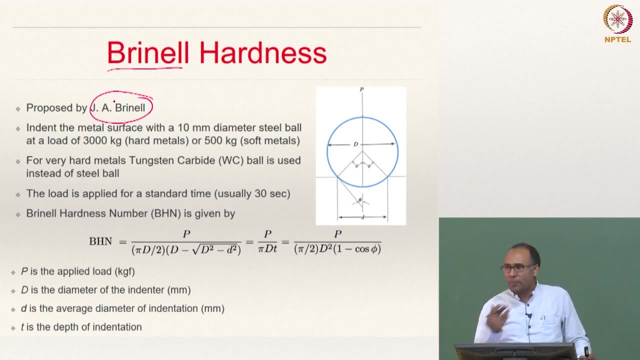 and see what is the depth of the indentation. And depending on the shape of the indenter you will have different tests. A Brinell hardness test uses a spherical indenter, a spherical ball, a steel ball as an indenter. So this diagram, this schematic represents, so this blue color one is your indenter and 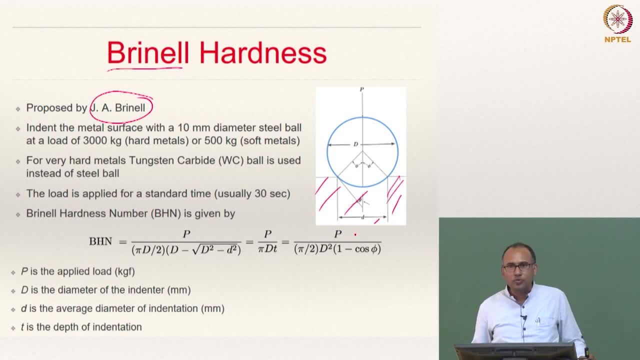 the bottom one. this guy is your material that needs to be tested for its hardness. And then you apply a load P and then measure what is the indentation depth, right? So this is the diameter of the circle that you would create on the surface, equivalent. 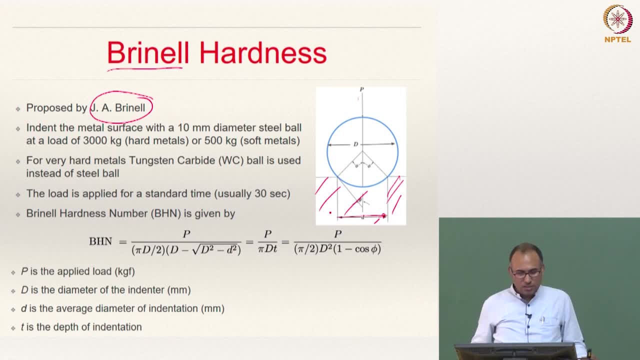 to the indentation area right. So the procedure is: you indent the metal surface with P, So you indent the surface with P. So you indent the metal surface with P, So you indent the metal surface with P. So 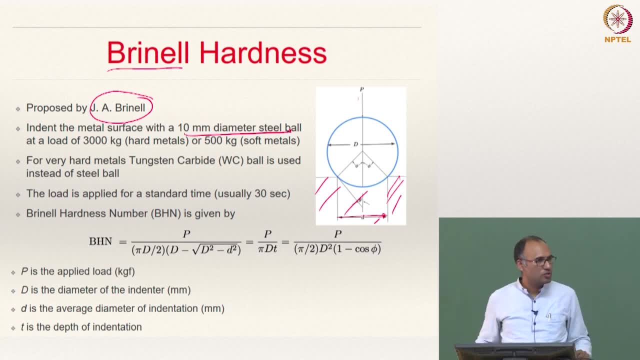 the procedure is: you indent the metal surface with P. So the procedure is: you indent the metal surface with P. So the procedure is: you indent the metal surface with a 10 mm diameter steel ball. This is the standard. the diameter of the steel ball is 10 mm for Brinell hardness. 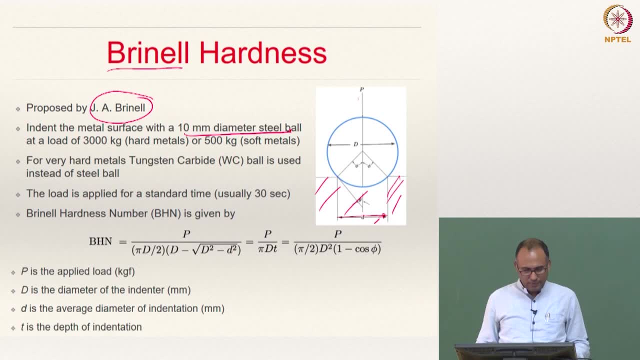 But if you want to change, you can change by following certain rules. And if it is a hard metal, you apply a load of 3000 kg, And if it is the soft metal, you apply a load of 500 kg. You decide what load you want to apply. 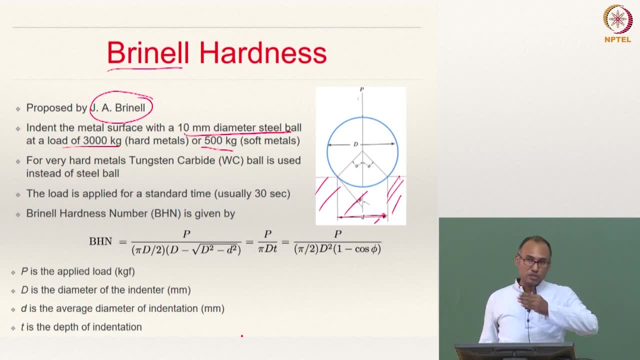 If the material is extremely hard. First of all, with respect to the material, the indenter has to be stiffer. right By applying load indenter should not deform. You are trying to measure the hardness of the surface And hence, if you are going to measure extremely hard surfaces, then steel may not be the right. 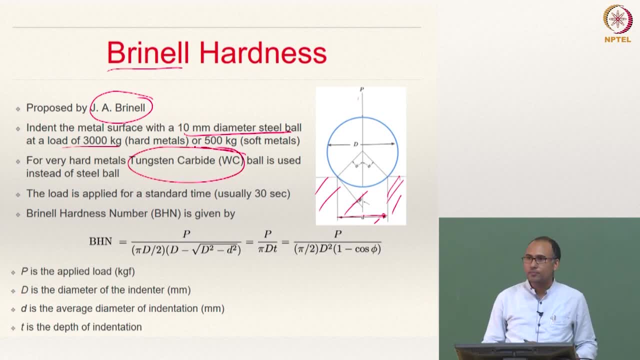 choice. In those cases, you will use tungsten carbide, right? If you are intending to measure hardness of surfaces which are harder than tungsten carbide, then you might want to use some other material procedure. okay, All right. 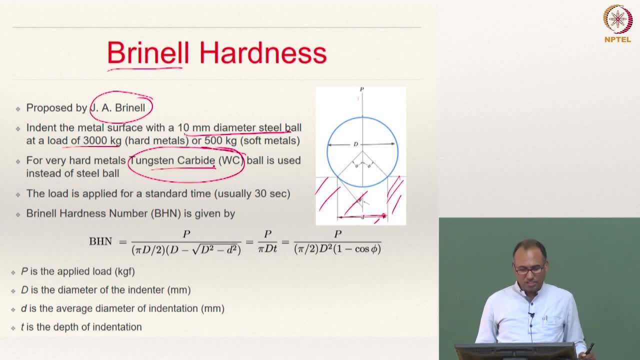 So for very hard materials or metals, tungsten carbide ball is used instead of steel ball And typically the load is applied for a standard time. The time is usually 30 seconds. You apply only for 30 seconds. Beyond that you do not apply any load. 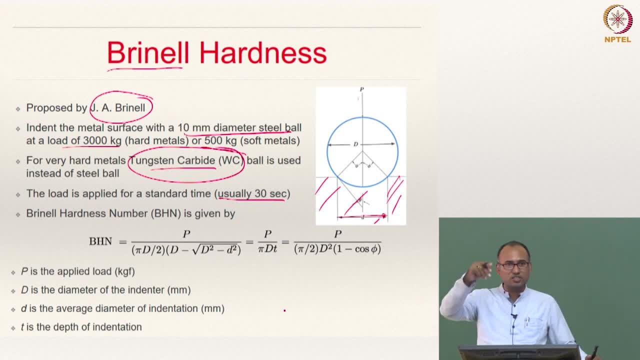 And then after 30 seconds you see what is the load, And then usually this load is applied not suddenly, but gradually, And then hold it. You hold that particular load for 30 seconds. That is what we mean. 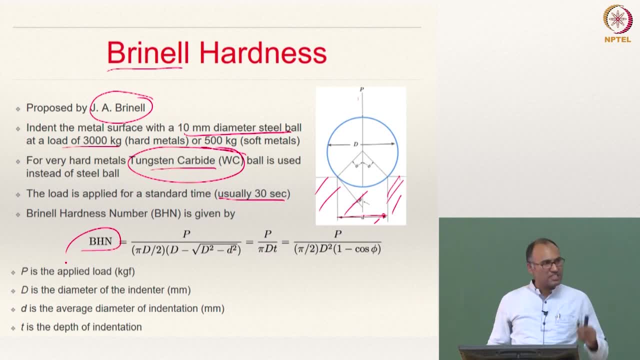 And the Brinell hardness number, that is the number that represents the hardness of this material, is some sort of stress measure, right, load by some area, right. So this is the Brinell hardness number formula. And then if you know this angle phi, then you know, if you know the diameter, so this: 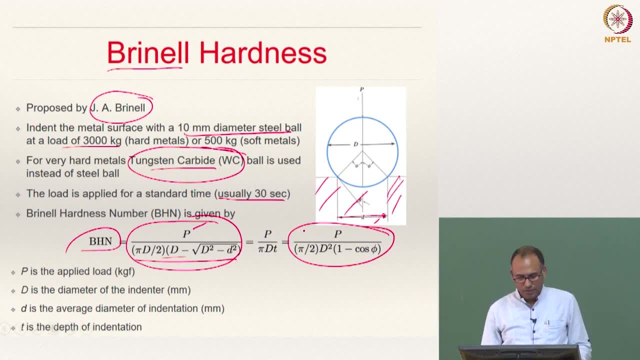 is how you calculate the Brinell hardness number And where p is the load applied, It is applied in kgf, D is the diameter in mm. That is important. This formula, when you are getting the Brinell hardness number, you are applying load in. 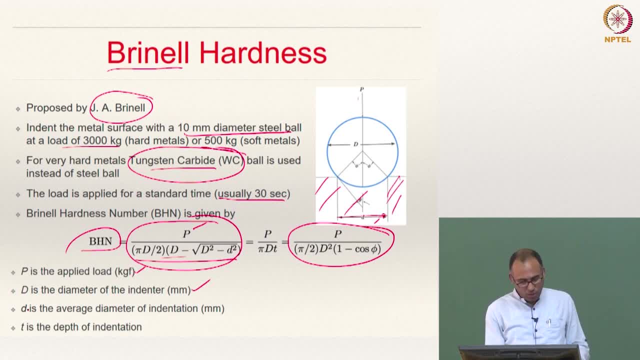 kg force. D is the diameter in mm. Small. d is the average diameter of the indentation. T is the depth of indentation. You can measure the depth of indentation. That is what you have. And now, if you want to use non-standard indentation, 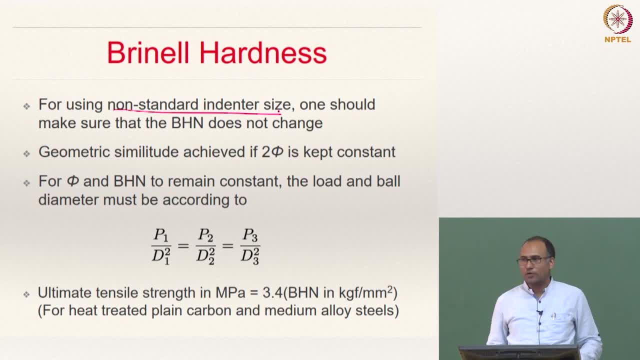 You can use non-standard indentation. You can use non-standard indentation, So you have to use the indentation size. You do not have 10 mm ball but you have, say, 5 mm ball. With 10 mm ball, what is the load that we have to apply? 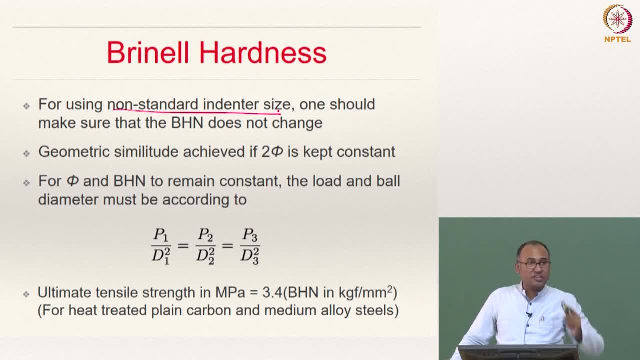 3000 kg. So you just need to ensure if you are changing the ball size, you also have to change the loads load that you want to apply according to this similitude formula. So if you change your D 1, so let us say D 1 is 10, then p 1 is 3000. 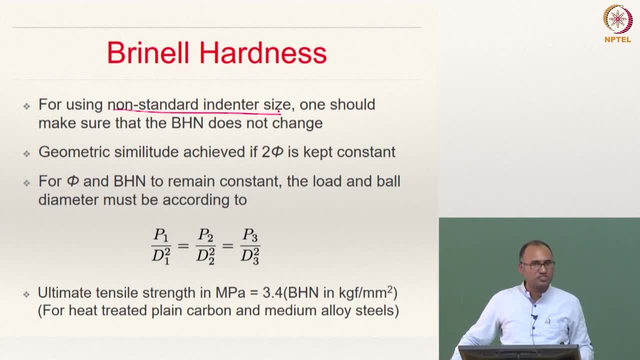 If you want to make D 2 to be 5, then accordingly you have to change your p 2 as well. That p 1 by D 1 square. you have to change that. So you have to take that p 1 by d 1 square and p 2 by d 2 square is what you need to maintain constant, because 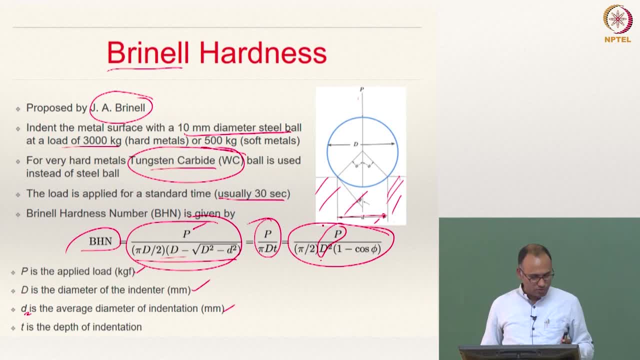 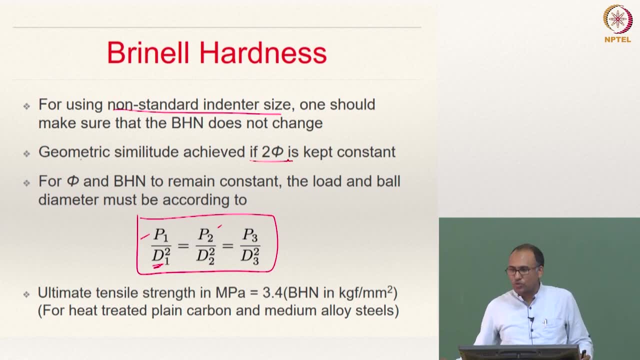 the Brinell hardness number is proportional to that And of course you. that is true when you are trying to make this. 2p is constant. that means you are getting the geometric symmetry And by measuring the Brinell hardness you can. 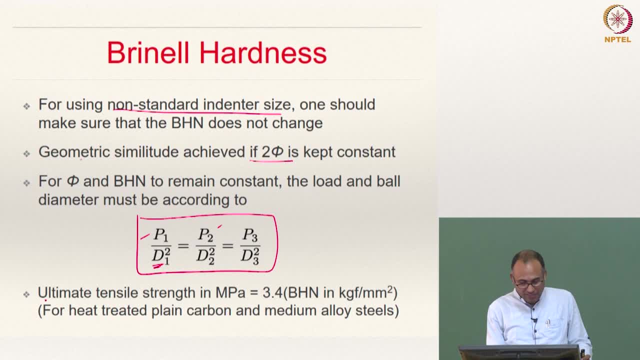 also sort of estimate the tensile strength of the material. It is only an empirical formula suitable only for plain carbon and medium elastic. That means if you know your Brinell hardness number in kgf per mm square from the previous formula, if you multiply that 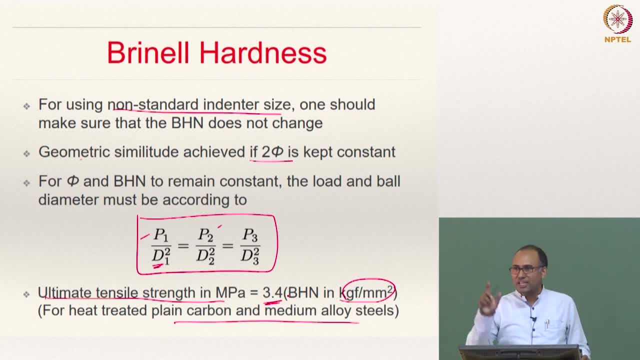 with 3.4, the number that you get is the ultimate strength of the steel in MPa. Okay, So if your Brinell hardness number is, let us say, 200, sorry, 70, 200 is too much So. 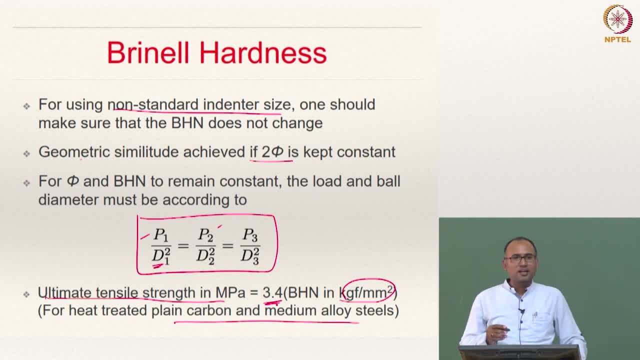 let us say not too much. Let us say it is 200, then 3.4 times 200 kgf per mm square. This should be in that unit. that is important. Then that is how much it is. 680, right, 680. 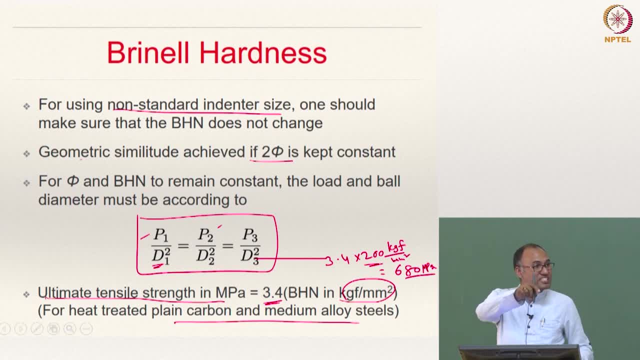 MPa, then the ultimate strength of that piece, The ultimate strength of that particular material, is 680 MPa. So the this is an empirical formula and hence please do not see the balance of units. The empirical formula work like that, right, Because on one side you have kgf per mm square, on the other side you have 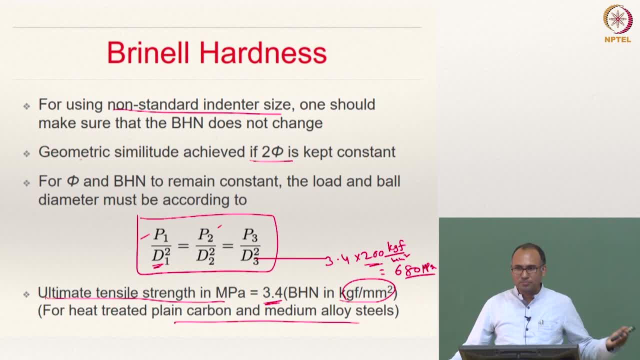 mega pascals. right, One is the metric system, actually not complete metric system. that is also a weird system, right? kg force and millimeters- they do not really go well, But that is how the standards are being used. So that is why this is important, So that 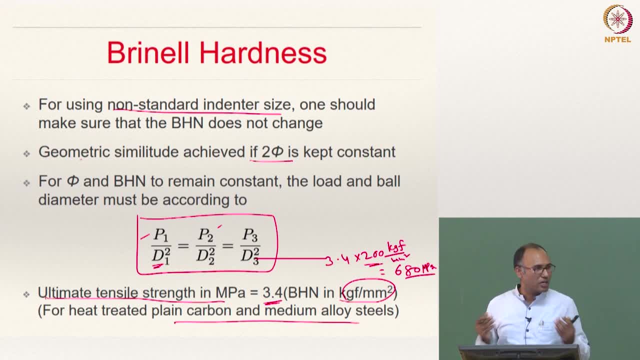 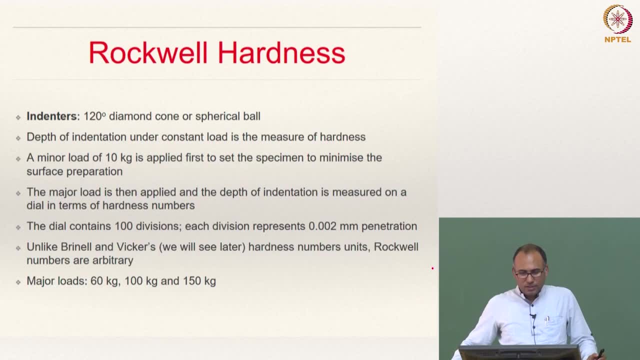 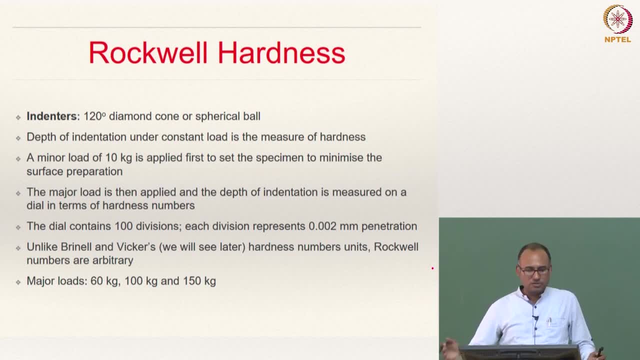 of watts that it uses. and that is basically the today is the average power of commutator system in the home factory. Yes, Yes. therefore, as you have seen by the situation, it does not work for other augments as an. karang, fizzy bonding cannot work. No, in general, we have found out that, alright, Just because in construction you can reason: Mỹ都是 Pick of its owner nature and you know even if the price for which you buy it is very much. 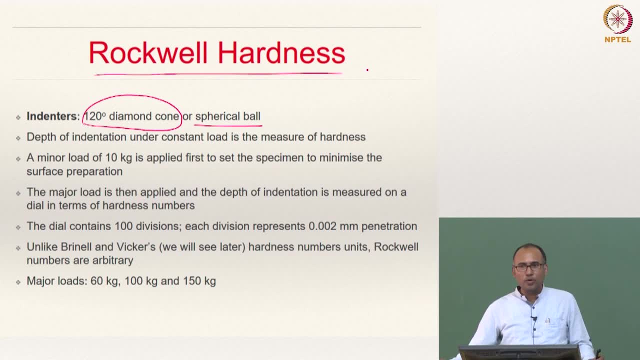 something called Rockwell hardness question. How does this guy work? You apply a constant load and measure the depth of indentation. That is the measure of your hardness, as usual. But how the test is to be done In this case. first you apply a minor load of 10 kg. You 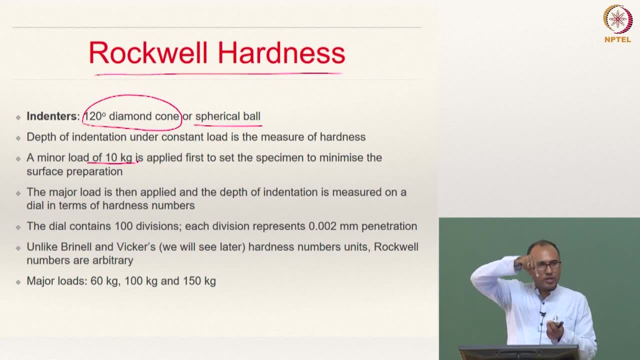 take the specimen and the indenter. First you apply a minor load of 10 kg just to prepare the specimen for the test, because there may be some surface scales and all So you want to get rid of them. So this 10 kg is used to get rid of these surface scales and you 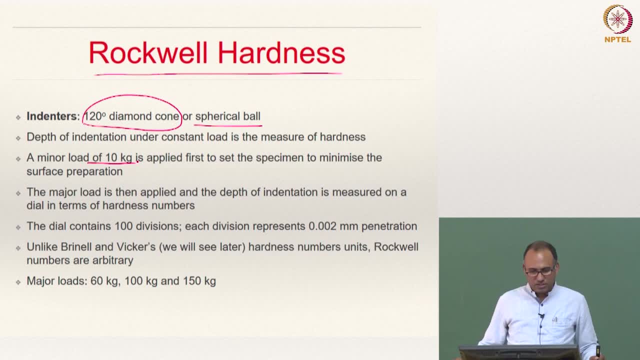 want to really measure the hardness of the real surface And then, once after applying this 10 kg minor load, then you apply the major load and the depth of indentation is 10 kg. So this 10 kg is used to measure the hardness of the. 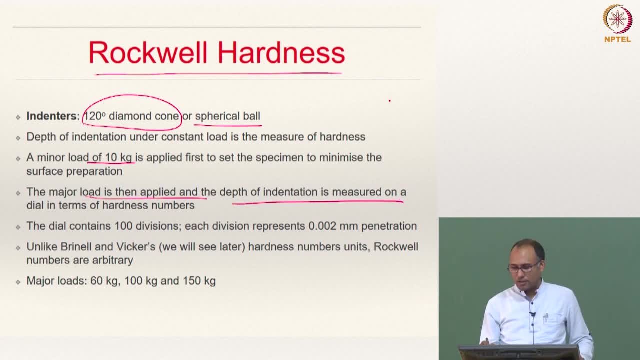 indentation is measured on a dial. So you have something like that with a dial gauge and here you have in your indenter and then you have specimen and then you press it and then you measure the depth by this dial gauge. This dial contains 100 divisions. Each division 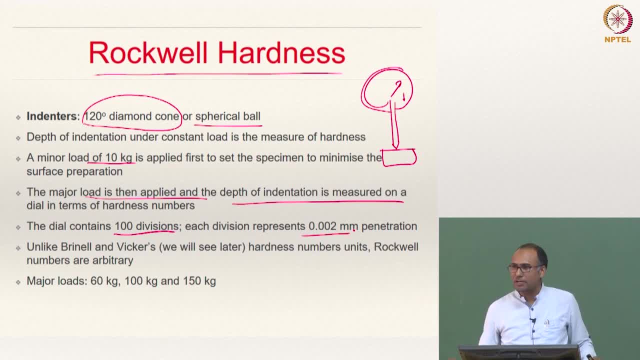 represents 0.002 mm penetration. Unlike. we will also talk about Vickers. But unlike Brinell and Vickers, the Rockwell hardness numbers are. they do not have a unit. What is the unit of Brinell hardness number? kgf per mm square, Whereas Rockwell hardness? 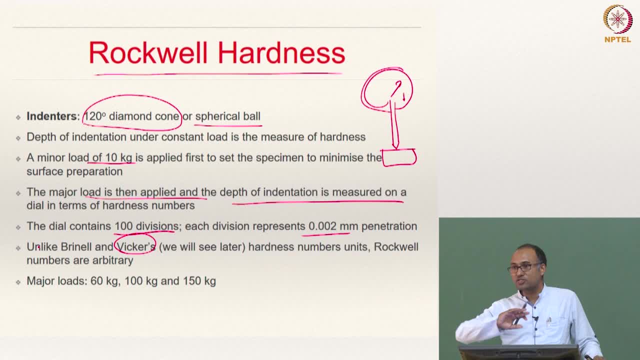 number is just only a number. If they are arbitrary there is no unit. So Rockwell hardness number, you will not report 0.002 mm, but you will report what is the scale the dial representing, what number the dial is representing on this scale. So we said: 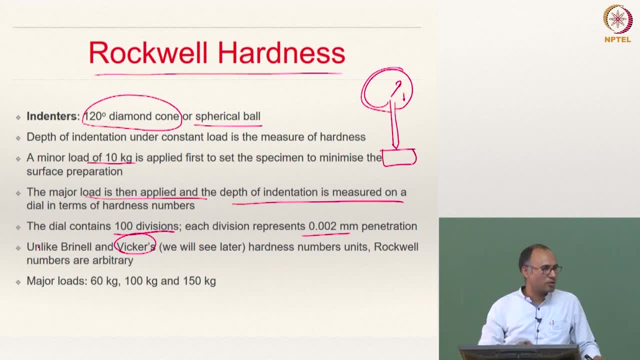 that the major load has to be applied. First a minor load of 10 kg and then a major load. The major load: what is the major load? It can be 60,, 100 or 150, one of them depending on the material. If it is a soft material, you will live with 60, little bit hard, 100,. 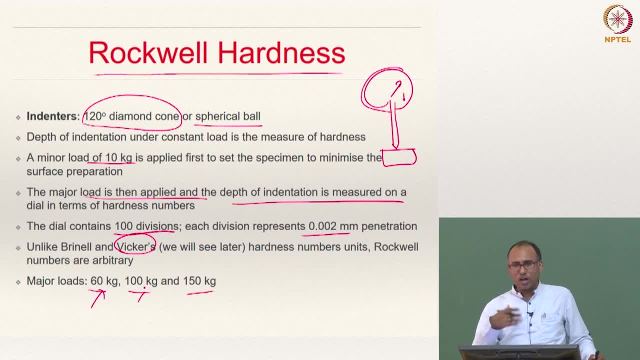 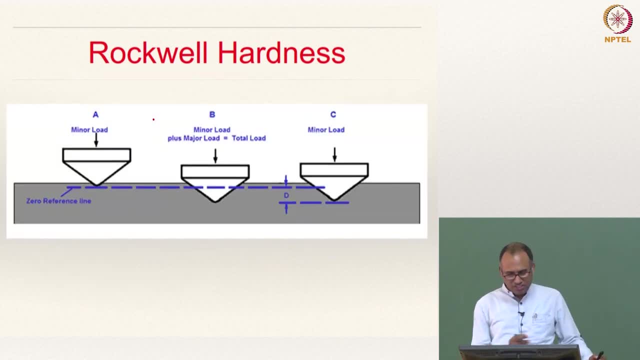 much harder- 150.. But Rockwell hardness test is primarily mainly done with 120 degree diamond cone, or sometimes you can also use spherical bone. So this is how you will apply. So you apply, you apply a minor load and then major load and then remove the major load. 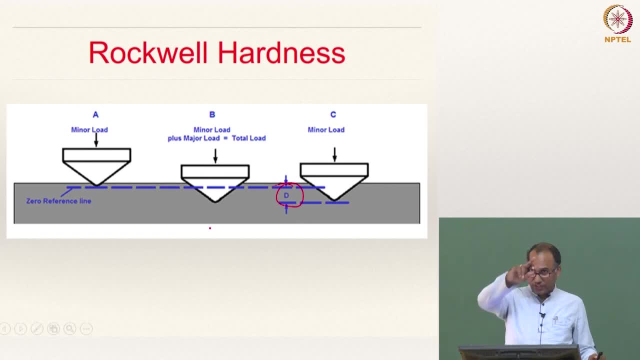 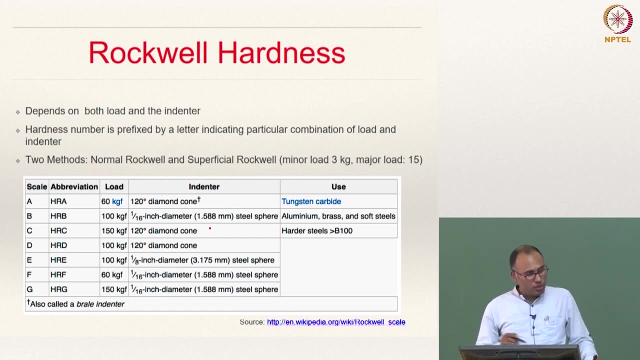 and then you measure the depth of indentation and that depth of indentation is shown on the dial. alright, So the Rockwell- different scales are available. So, depending upon which scale are you using, you have to mention Rockwell A, Rockwell B, Rockwell C, D, E, F, G. So 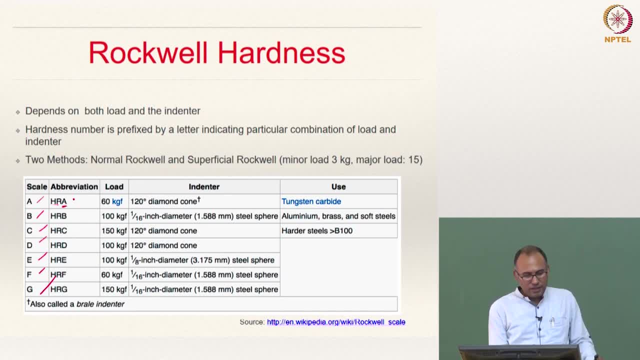 Rockwell hardness on scale A. what is the meaning of that? If you are saying that by HRA is some number, that means I am applying. I am using a 120 degree diamond cone indenter and the load is 60 kg F. That is the meaning of Rockwell scale A. If I say Rockwell scale, 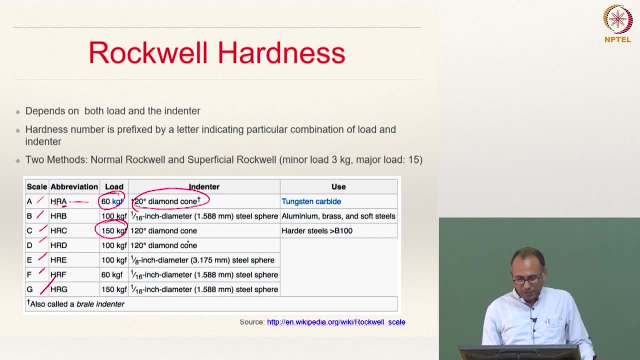 C. that means I am applying a load of 150 kg force and 120 degree diamond cone is my specimen like that. So I am applying a load of 150 kg force and 120 degree diamond cone is my specimen, So 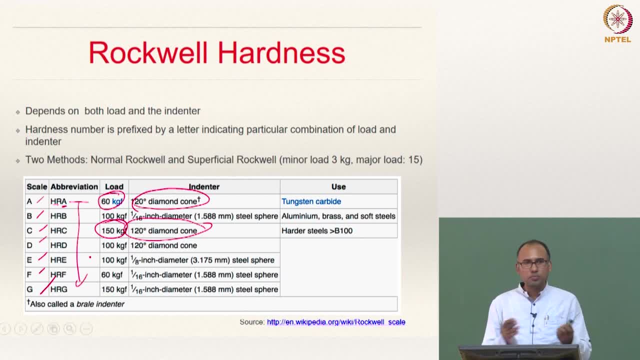 there are different scales that are defined just to represent what is my geometry of the indenter and what is the load that I am applying. So whenever you are, whenever you are reporting the hardness number from Rockwell hardness test, you have to report what kind of scale. 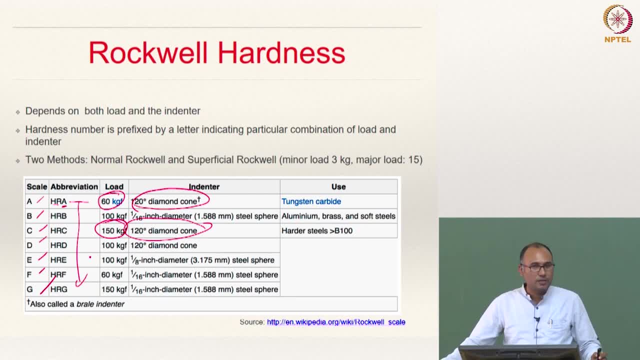 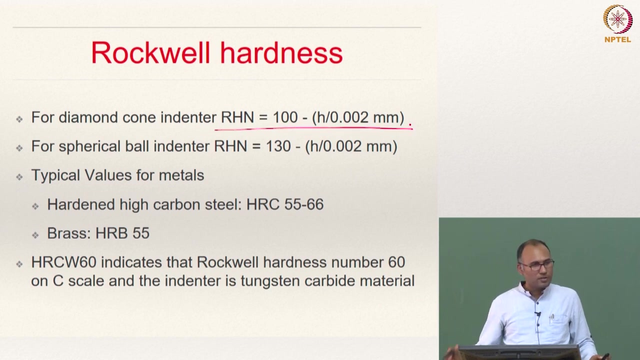 have you used? Is it HRC, HRB or HRA? And unfortunately you cannot write a direct correlation from Rockwell to Brunel. You do not. you do not have an empirical formula that relates Rockwell to Brunel. All right, So the way that Rockwell hardness number is calculated with this RHN equal. 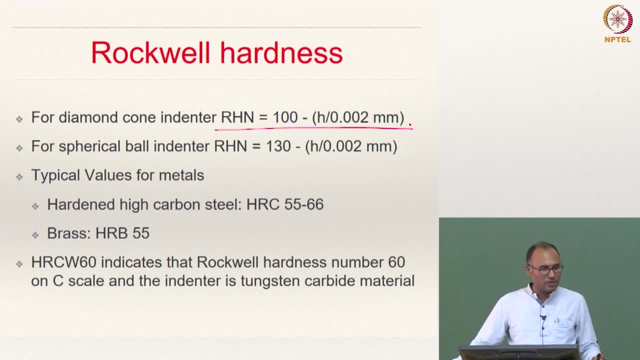 to 100 minus H by 0.02 for a diamond cone if it is spherical, spherical ball. this is how Rockwell hardness number is represented. So the typical way that you would if you are looking into standards, the way that you will see hardness number to be HRC typical. 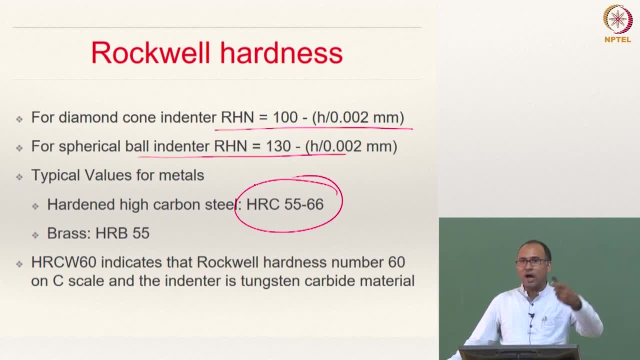 is 55 to 66.. It is actually a hardened, So the hardness is relatively higher. That is what we mean by this right. HRC 55 by 55 to 66 is the Rockwell hardness number for high carbon steel. For brass it is HRB. Please see the pay that. pay attention, Both of. 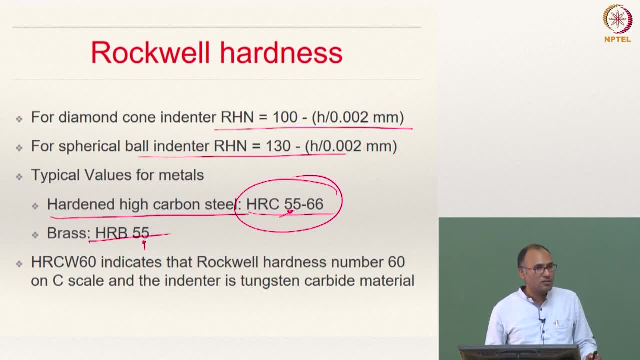 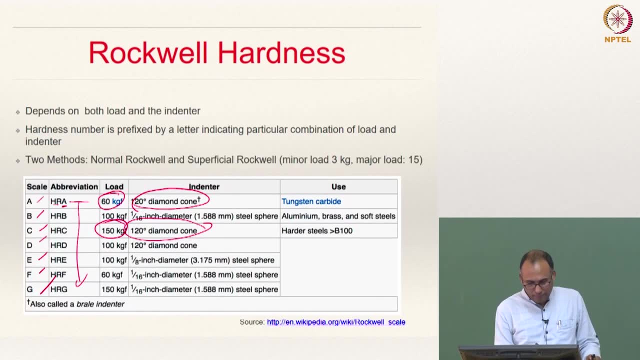 them are giving you almost same dial scale, but this is C and that is B. So what is C? Where C and B go back, B is only having 100 kg force, Whereas C is having 150 kg force. And this specimen, the indentry steel sphere, and here it is 120 degree diamond cone And 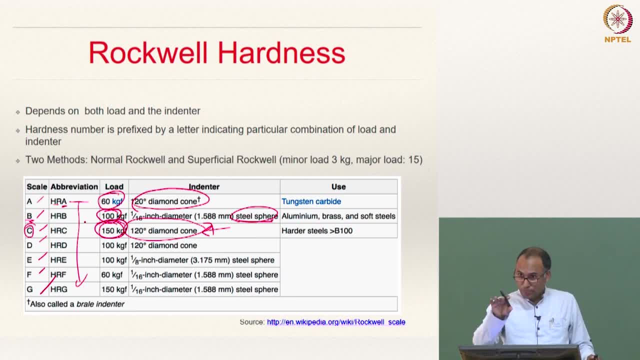 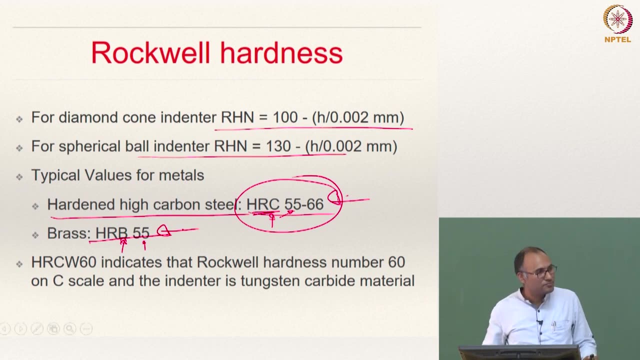 hence, HRC 55 is actually more severe indentation depth than HRB 55.. Can you see that? And that is the reason why you need to specify what is my scale. OK, Thank you. So that is why you can say that this is actually harder than this case. is that clear? 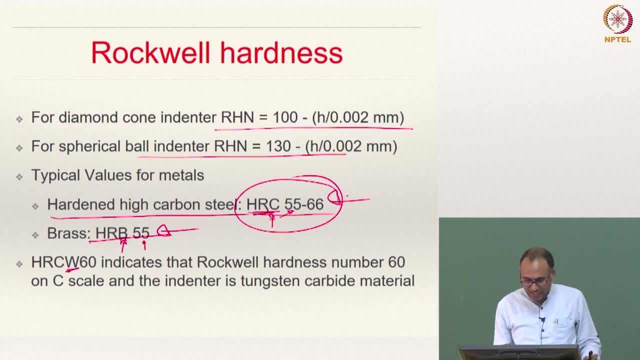 So HRCW? if you say HRC, that means my indenter is a steel bond. If I am putting HRCW 60, that means my indenter is not steel but tungsten carbon. The W represents the material of the indenter. 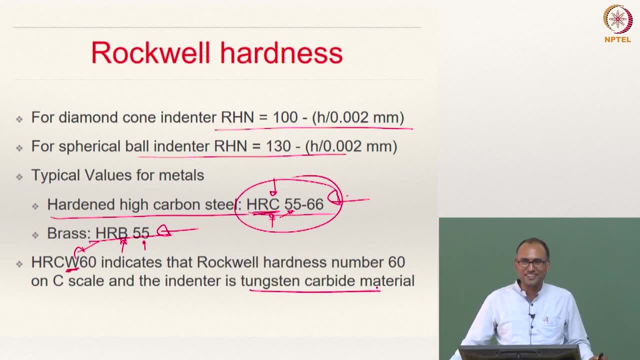 Any questions? There cannot be any questions here. it is only an information, just to remember. you do not have to remember the numbers, you just need to remember how the designation is made. If I say HRCW 60, then you should be able to say that it is the indenter is a tungsten. 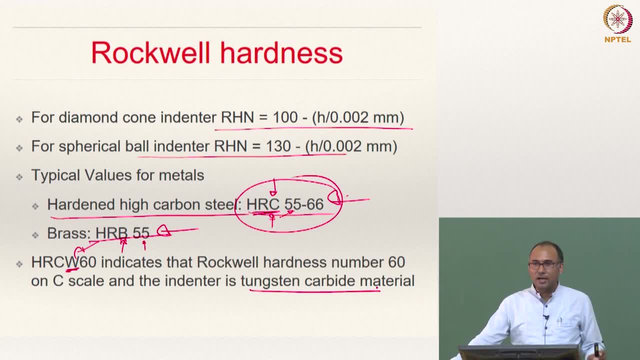 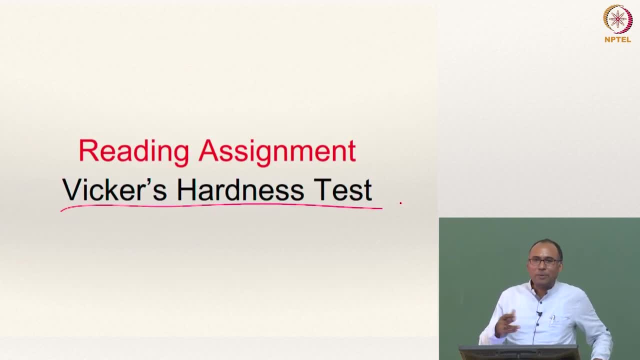 carbide indenter, not a steel indenter. and it is not a spherical indenter. it is a steel indenter. It is a 120 degree diamond cone indenter. This is diamond pyramid. The indenter is different in a Vickers hardness test and the way the Vickers hardness test. 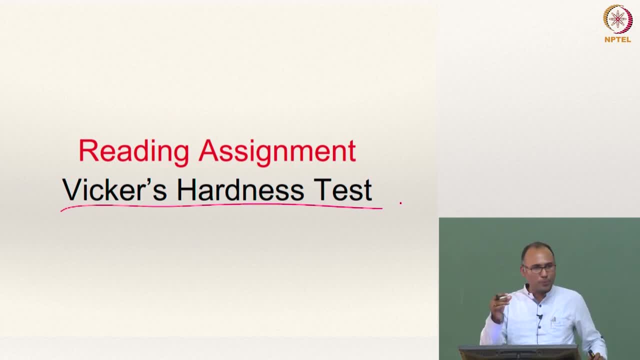 works is similar to Brinell hardness test. it also reports the load by area, unlike Rockwell hardness So many times you might. actually, you will do an experiment In ME lab next semester. there you will measure hardness of a surface using Vickers hardness. 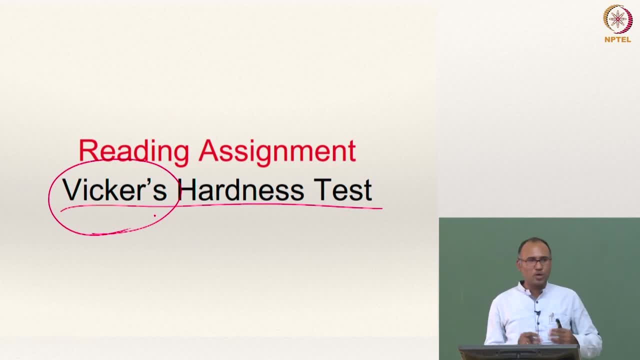 test. So then you need to know the geometry, and then from the geometry you will be able to calculate what is the hardness number of the hardness value of this material. We in the lab we have the Vickers hardness test, and if somebody else comes up with something, 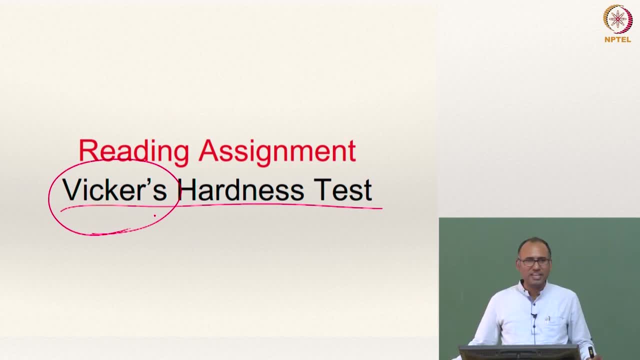 else and which is better than these things? probably that hardness test come in. There is no. this is something that people have evolved over the years and you know the numbers. now, If you go to a catalog and you have, you know the numbers and then you say that my hardness. 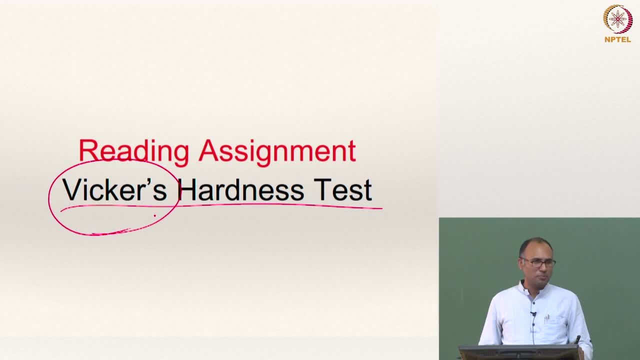 is this, And if you want to come up with your own standard, welcome, but make sure that world is okay with that as well. That is how these standards work: Rockwell hardness, Rockwell hardness, Rockwell hardness. 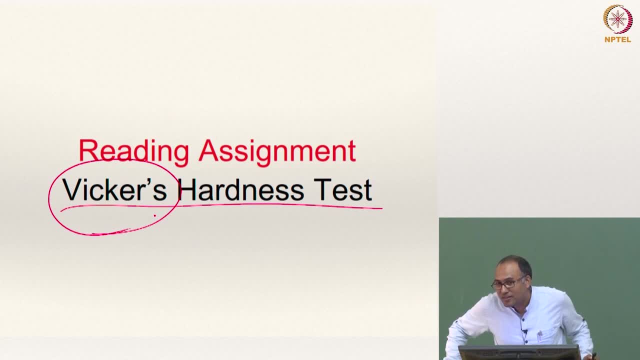 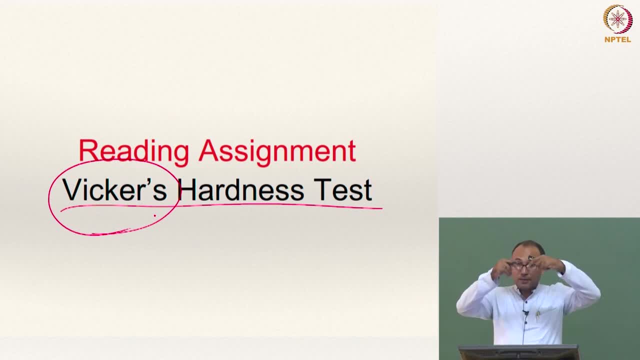 So the fact that the indenture shape is different, the local stress state is going to be completely different, right? If you are taking a material and if you are using this kind of an indenture, this value, this kind of an indenter, the local state of stress below the indenter is going to be. 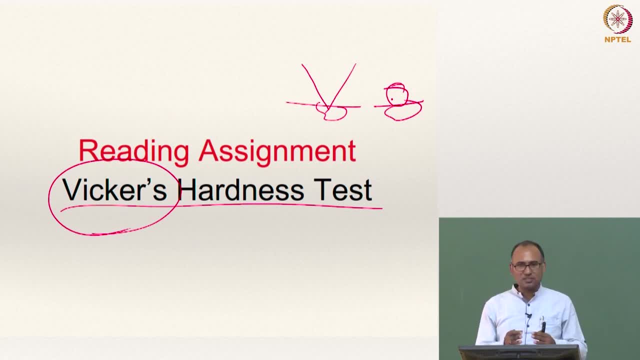 very different. The stress state is going to be much more severe in this case compared to here and so on. So it is to my knowledge. I do not think we have any direct correlations from one scale to another scale, but you can sort of make an assessment that, if I the way that you 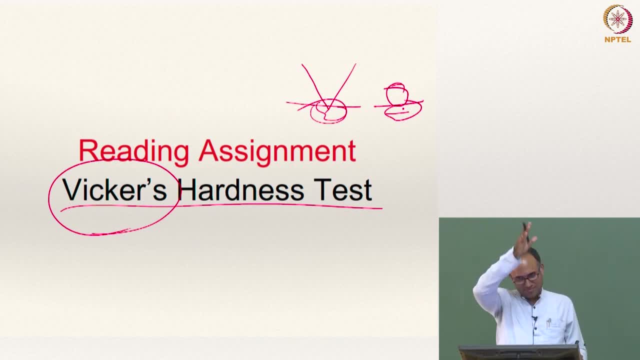 need to do is you need to do the tests on the same material using Rockwell A and Rockwell B, C, D, and then try to see an empirical form. In principle one can do that. I do not know if such things exist. 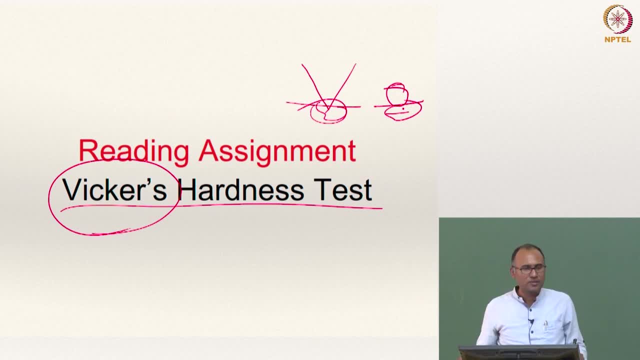 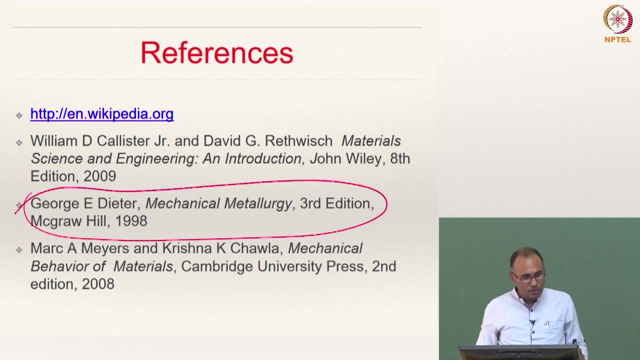 May be they are there, but to my knowledge I do not know if they exist. okay, You can actually go back and verify. it is a good exercise, all right, Any other questions? Good, So, So this is the textbook that I was referring to. 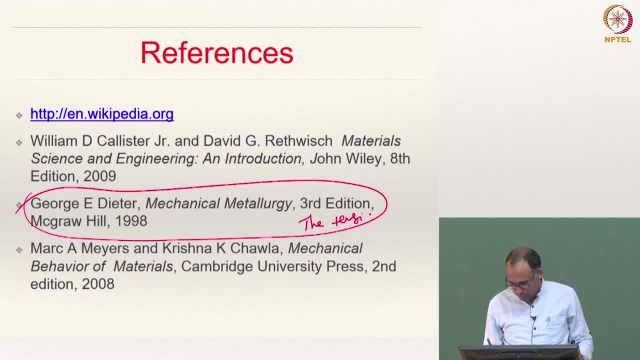 You have to read the chapter the tension test. all right, So with that we close mechanical properties. You have any questions?